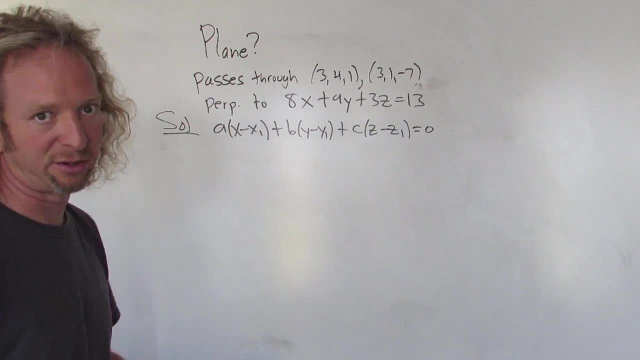 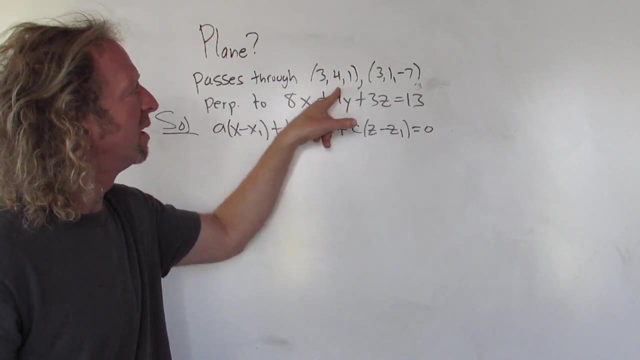 on our plane And then a, b, c, that's going to be our normal vector. So that's what we need. So we already have the points, we just need the normal vector. So we're given two points on the plane. So, given two points, we can always find a parallel vector. So let's go ahead and do that. 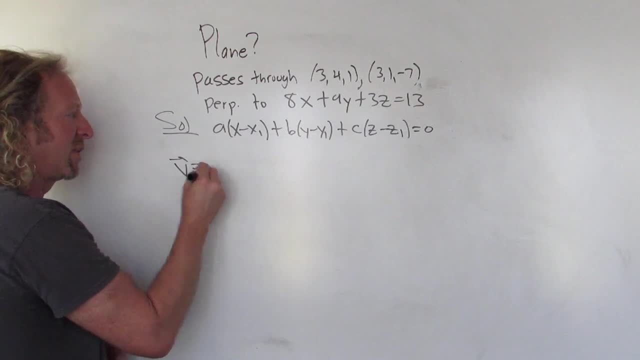 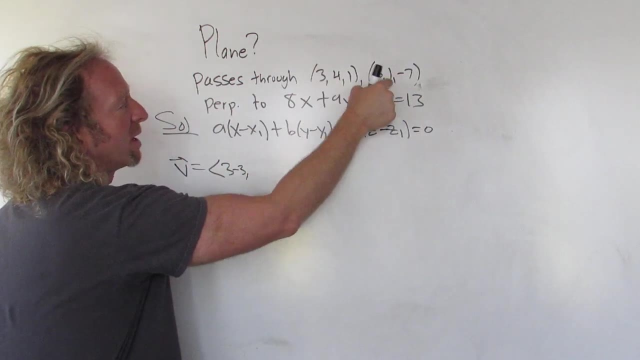 first, and then we'll read this. So let's write down our parallel vector that we have. So 3 minus 3.. I'm going to skip some steps here. No, I won't. 1 minus 3,, 4 minus 1, and then 1 minus negative 7.. So what are we doing? We're finding a parallel. 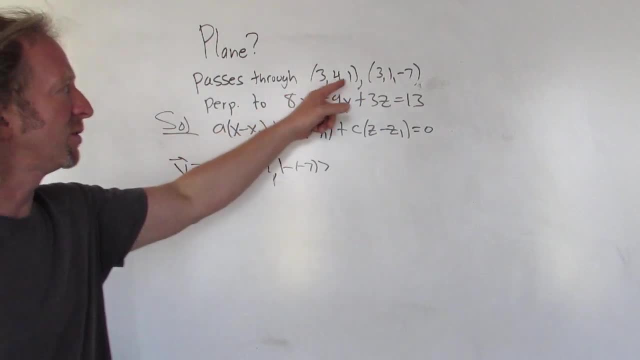 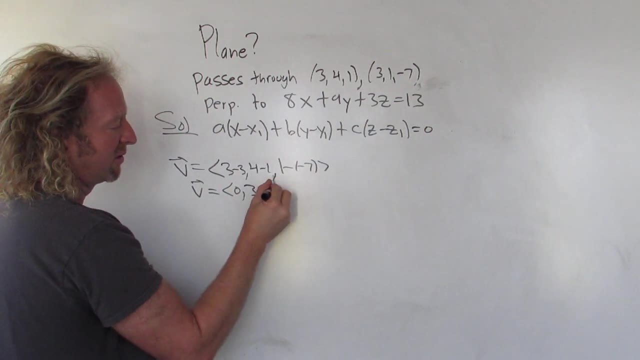 vector y, We'll need it. And plus I mean whenever you're given two points, you probably have to find a parallel vector. So this is 0,, 3, and then 1 plus 7 is 8.. So this vector is parallel to our plane. 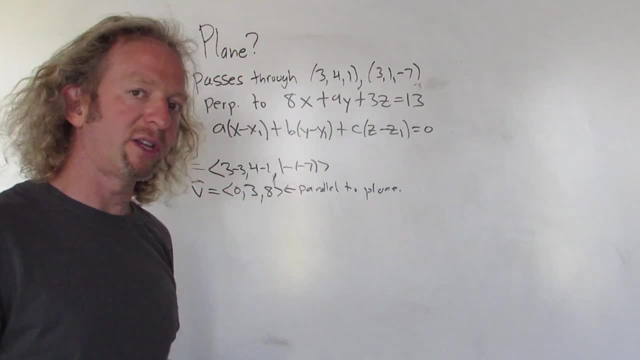 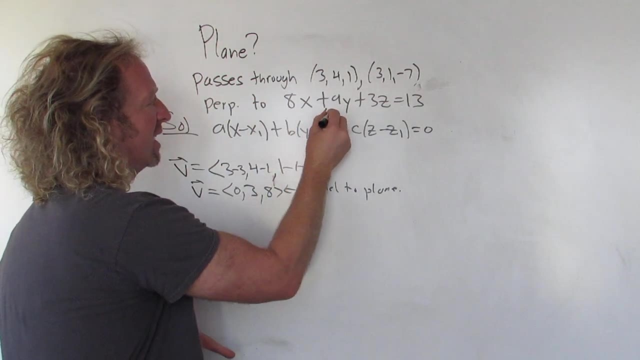 Okay, now we're told that our plane is perpendicular to this plane, So we have to think about that. right, This vector here? 8,, 9,, 3, this is the normal vector for this plane, right, This vector. 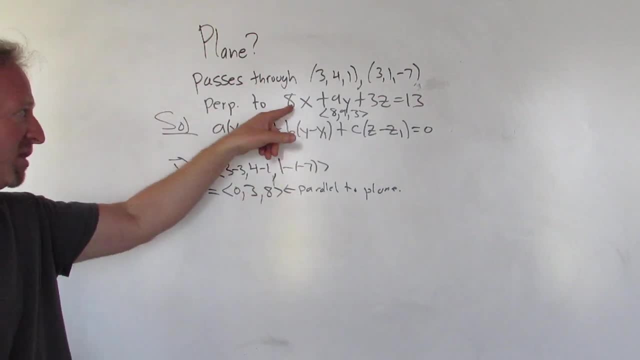 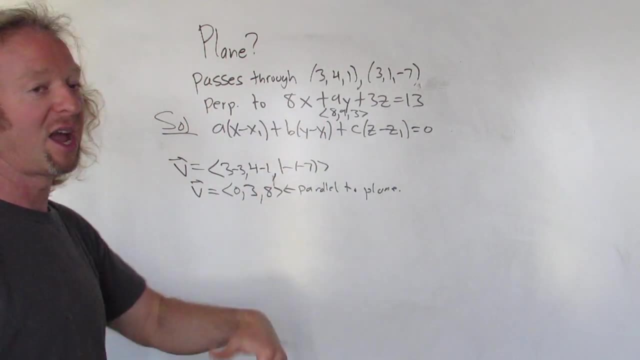 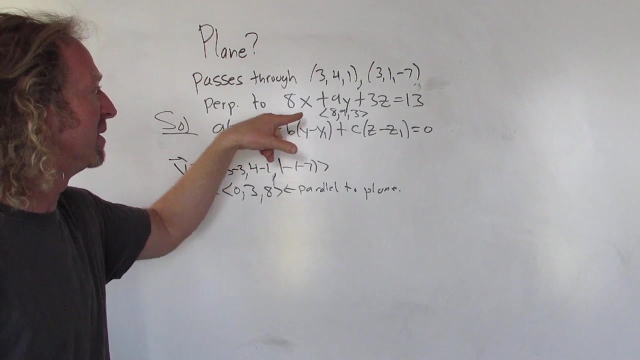 is perpendicular to this plane. So our plane is perpendicular to this plane. This vector is perpendicular to this plane. Therefore, our plane is parallel to this vector. Again, our plane is perp to this guy. This vector is perp to this guy. Therefore, our plane is parallel to this. 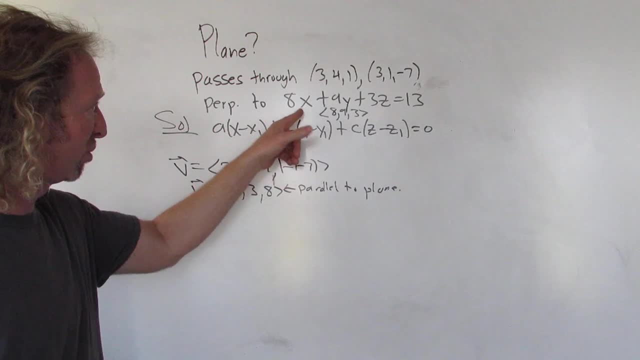 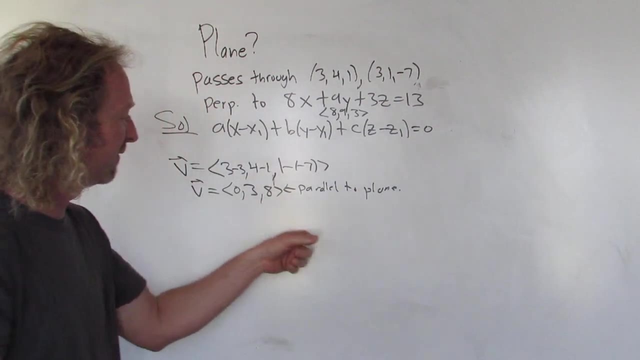 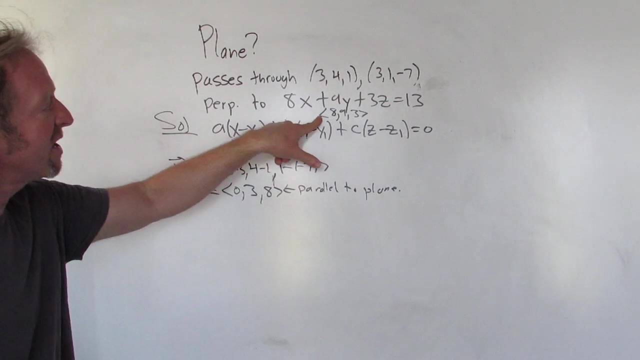 of the board as this plane. If the board is this plane, our plane is perp to it, this vector is perp to it. oh look, they're parallel. Again, if this board is this plane here, then our plane is perp, this vector is perp. oh look, they're parallel. So this vector is. 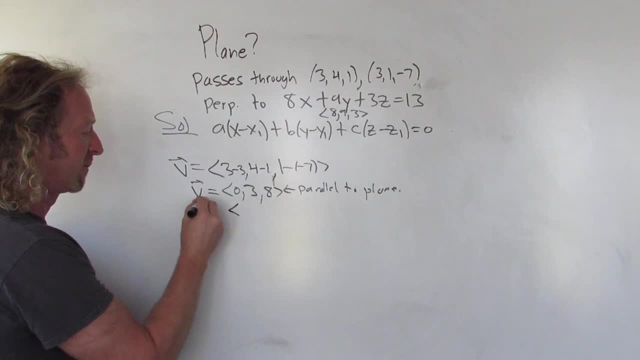 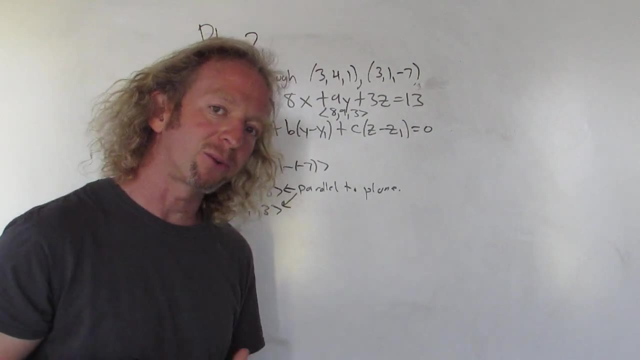 parallel to our plane. So we have another vector- I'll call it, u just give it a name- 893, and this is also parallel to our plane. We have two vectors that are parallel to our plane, so we can find the cross product to find a vector that is normal to our plane. 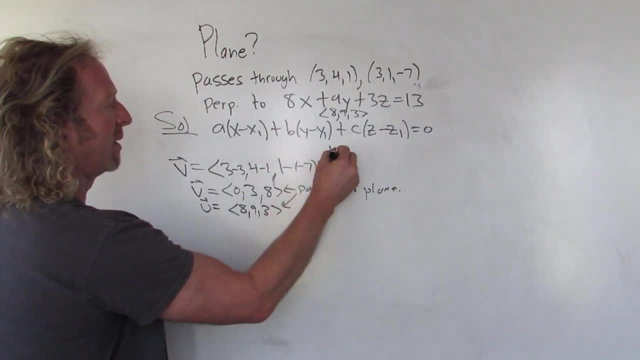 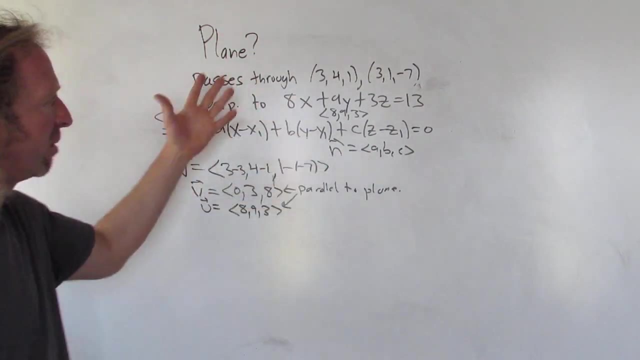 which is what we need, which is our n, which I didn't write it down, But n is abc, That's our normal vector. So we'll take the cross product of these two, that'll give us n, plug everything in and we're done. So let's do it. let's do v cross u. Now, it doesn't matter. 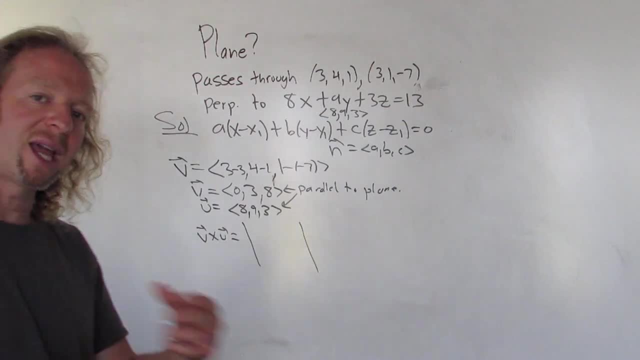 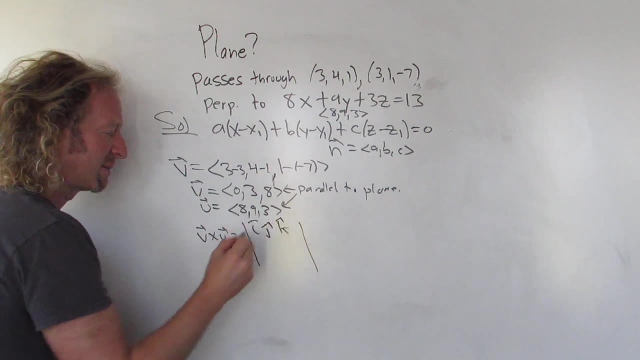 which order you do it in, you will get a different answer for the cross product, but at the end you'll get the same answer. So first you write down ijk and then you write down the little hat- sometimes I forget the hats guilty- And then v is 038,, so 038, you always. 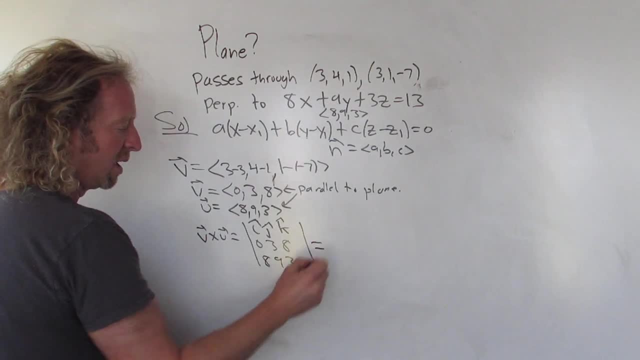 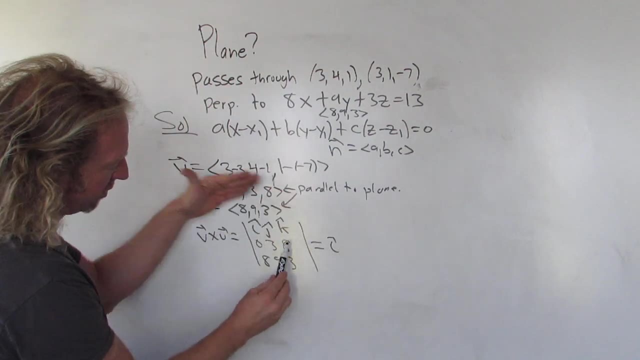 write that one down first, and then u is 893.. And when you're doing the cross product it's always plus minus plus, so it's ihat. then you cross these out. so 38,, 3893,, 3893, so. 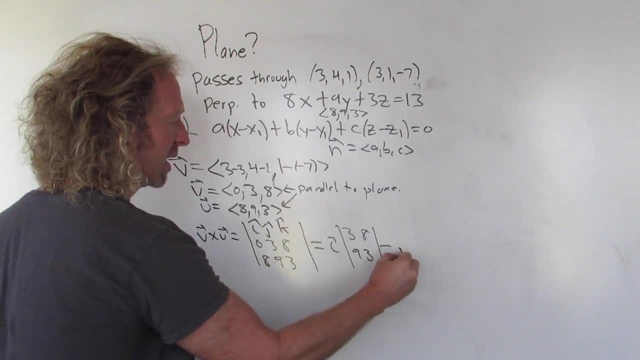 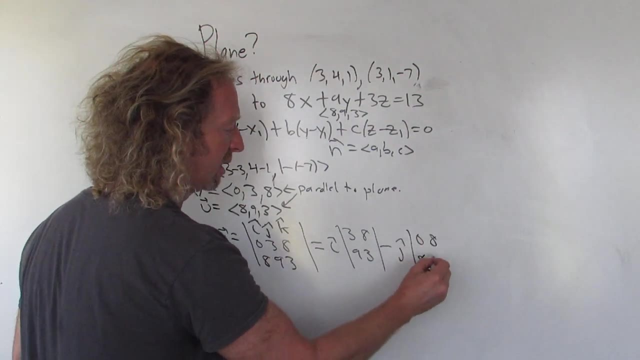 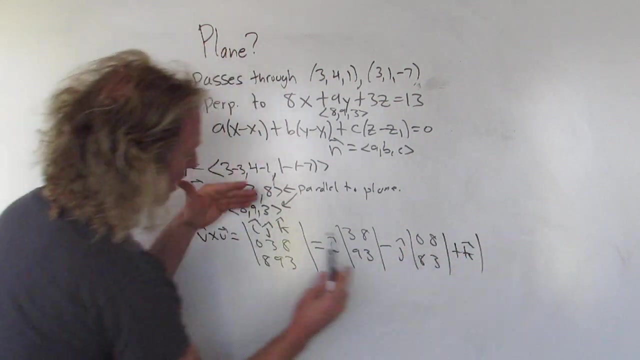 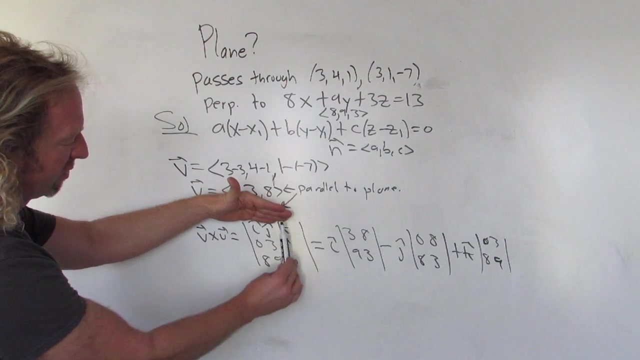 3893, and minus jhat. it's always plus, minus, plus, and you cross these out, so 0883,, and then you cross the corresponding row and column and then boom and then khat. so plus, so plus khat. 0389,, so 0389,, 0389, like a phone number, 0389.. Let's check that, so ihat. 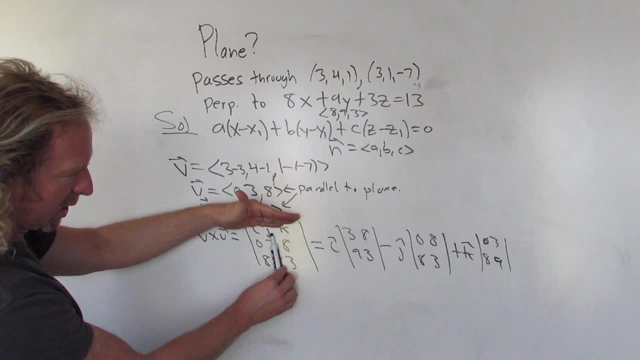 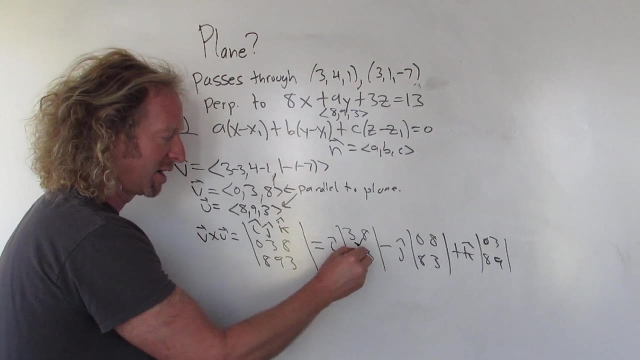 oh looks okay. jhat looks okay. khat looks okay. okay. Alright, now we just work it out. So you multiply this times this and you subtract this times this, So it'll be: ihat jhat looks. 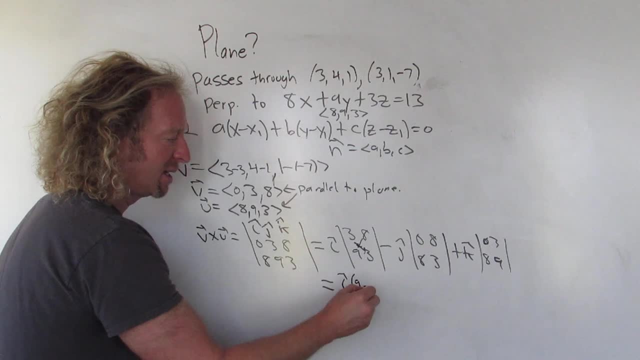 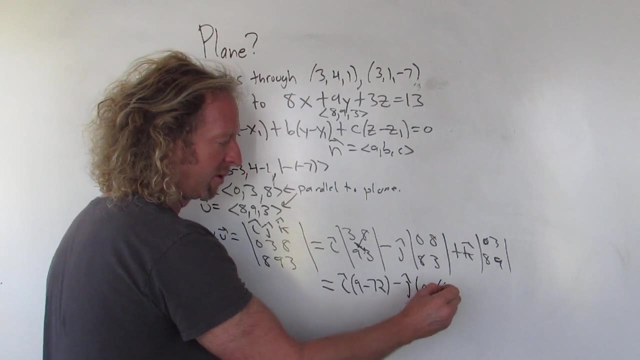 okay, khat looks okay. So we have that. 9 minus 8 times 9 is 72, some big numbers here. minus jhat, that's gonna be 0 minus 64, right, because 0 times 3 is 3,, 8 times 8 is 64, and then 0 times. 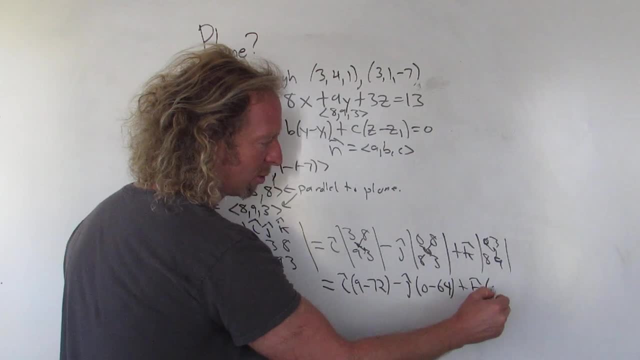 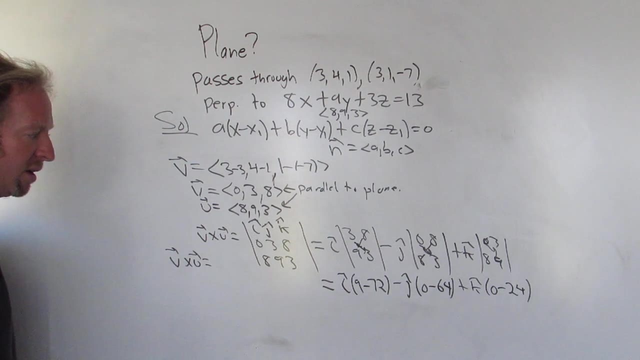 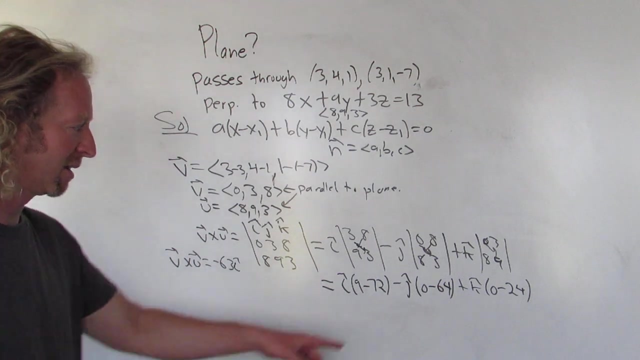 9 is 0, so plus khat, 0 minus 24.. Tough problem, So I'm gonna write it again over here. so b cross u. So let's see 9 minus 72, that's gonna be be negative 63, negative 63, and negative 63. i hat plus 64. j hat big numbers, feels. 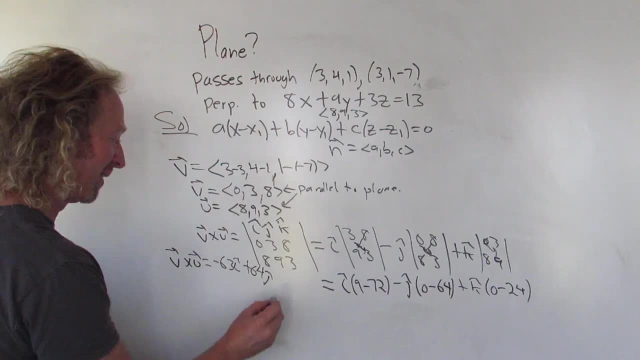 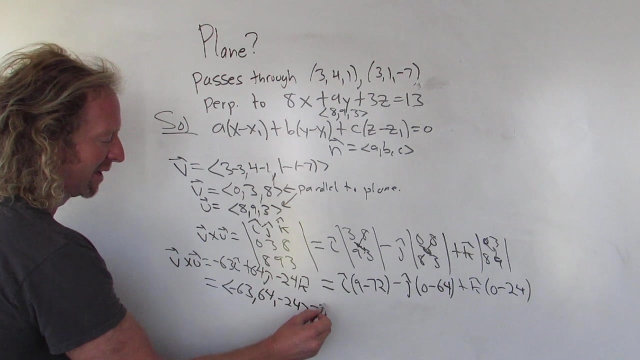 really wrong, but hopefully it's not minus 24 k hat. no, it's not wrong, this is totally correct. so there is our normal vector. so negative 63, 64, and negative 24, really really big numbers. that's our n, that's our n. so to finish, we'll just plug everything in here.